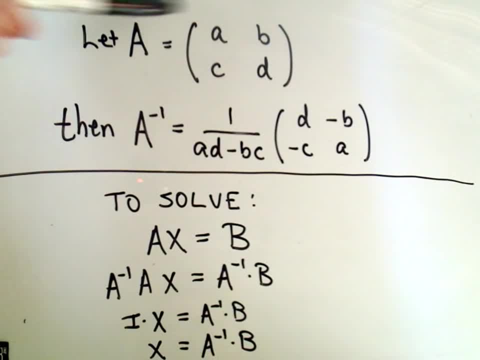 So remember for a 2 by 2 matrix A, B, C, D. to get the inverse, you take 1 over A D minus B C. that's the determinant. And then you flip the A and the D values and you change the sign on the B and the C values. 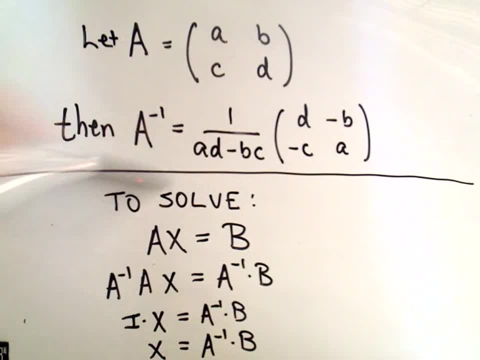 And obviously this will not work if the determinant A, D minus B, C equals 0. But to solve the idea is: we have a matrix equation, so AX equals B. we'll multiply both sides by A inverse. The left side will just be left with X. that's what you're trying to solve for. 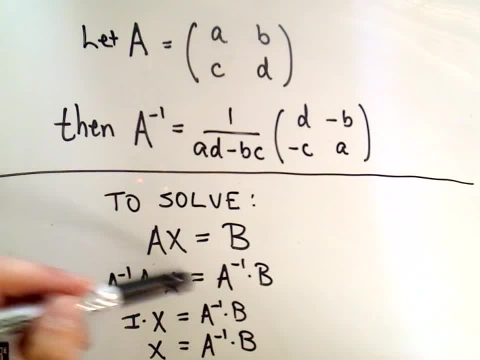 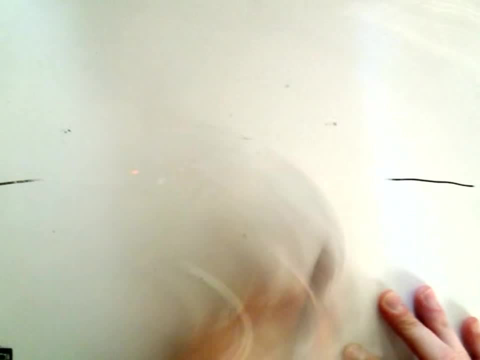 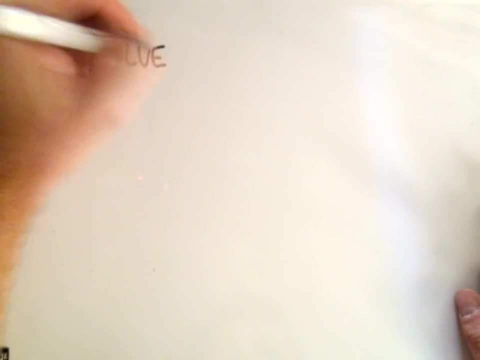 So basically it says: to get the solution to this equation, all you have to do is multiply the right side by the inverse. So let's do at least one or two here, hopefully. So let's solve this system. So we're going to do: 3X plus 5Y equals negative 1, and then X minus 2Y equals 4.. 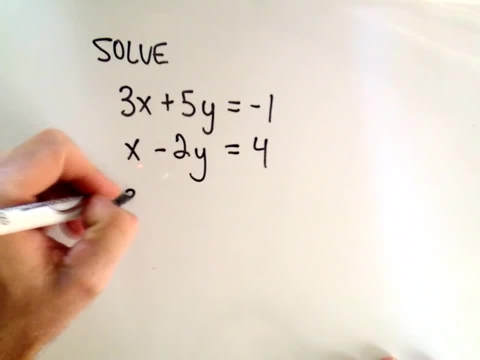 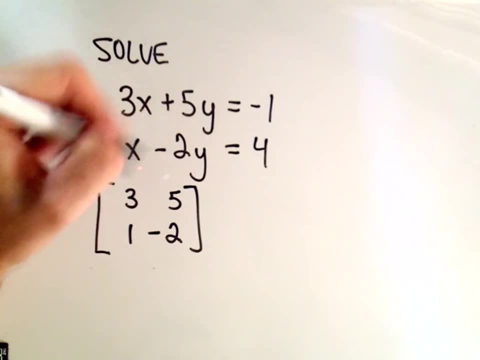 So again, I can write this as the matrix equation: 3,, 5,, 1, negative, 2, the coefficients on my X's and my Y's, So 3X plus 5Y, 1X minus 2Y. 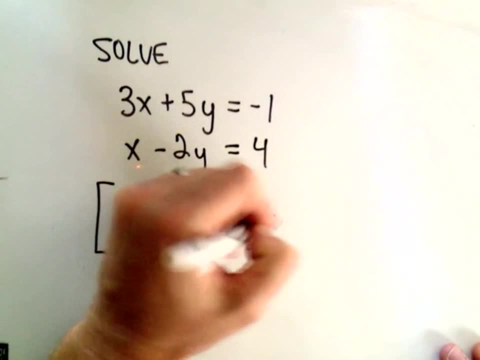 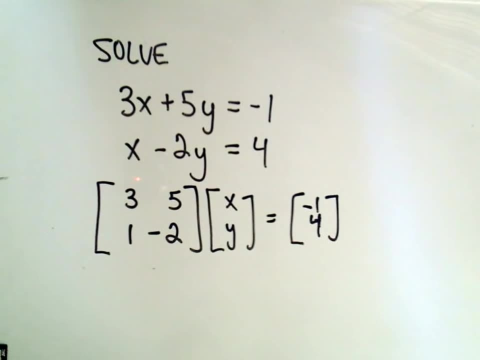 I can multiply that by XY and that's going to be equal to negative 1, 4.. Okay, in terms of what we just had, this is that matrix equation AX equals B. So now, if I can just multiply both sides by A inverse, 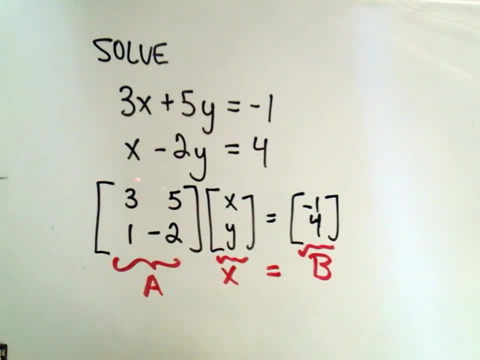 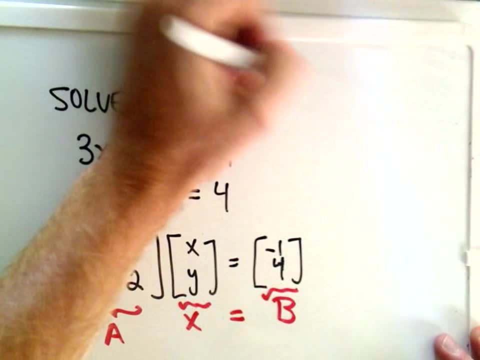 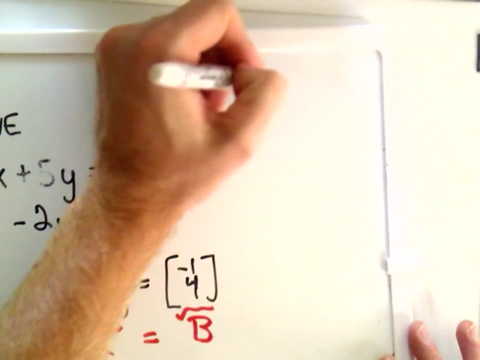 then I'll get the solution to this system. Okay, well, the first thing is to find A inverse. Okay, so we can use our formula, though, Again, 1 over AD minus BC times, we flip the diagonals and then change the other diagonals. 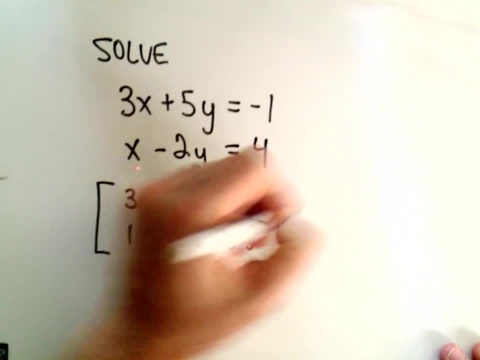 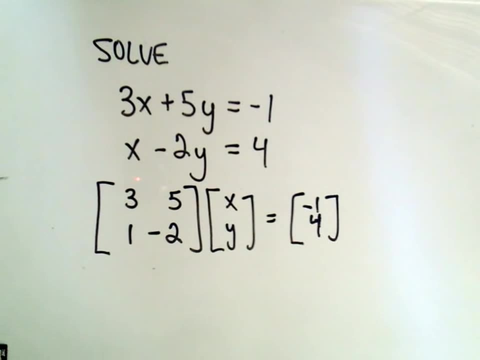 I can multiply that by XY and that's going to be equal to negative 1, 4.. Okay, in terms of what we just had, this is that matrix equation. This is the matrix equation: AX equals B. So now, if I can just multiply both sides by A inverse, then I'll get the solution to this system. 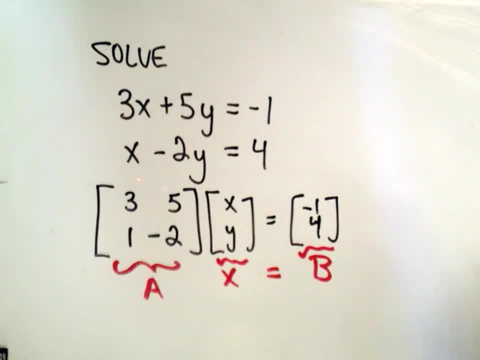 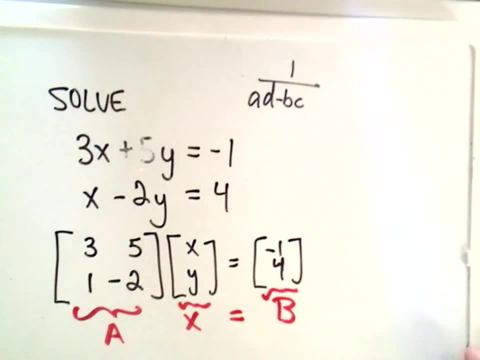 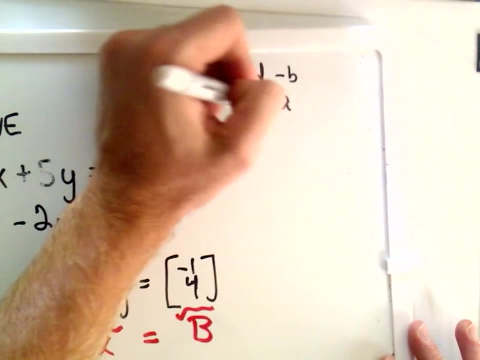 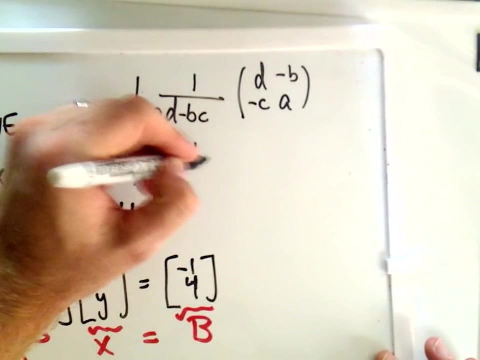 Okay. well, the first thing is to find A inverse. Okay, so we can use our formula, though, Again, 1 over AD minus BC times, we flip the diagonals, change the other diagonals, So in this case our inverse is going to equal. okay, so here's matrix A, down here in the corner. 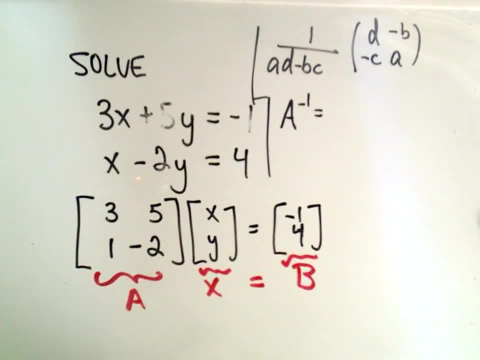 Maybe we'll just see if we can't fit it all in here. So it says A inverse is going to equal. so I have to take 1 over 3 times negative 2, and then it says subtract 1 times 5.. 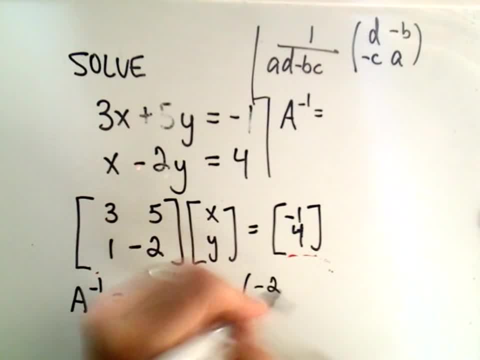 And then I have to flip the 3 and the negative 2, so I'll get negative 2, 3.. And then I have to change the signs so I'll get negative 5, negative 1.. And let's see if we simplify this down, it looks like you get negative 6 minus 5,. 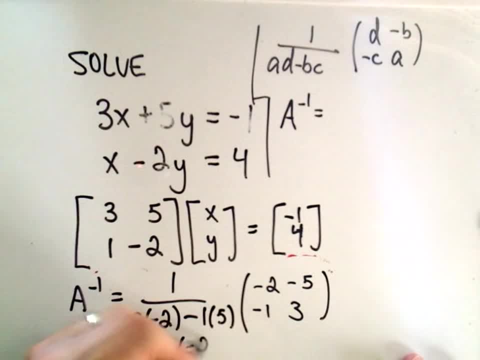 which is 1 over negative 11, and then negative 2, negative 5,, negative 1, 3.. Okay, so it looks like our inverse matrix. We could go ahead and multiply it. We could multiply this out and maybe clean it up a little bit. 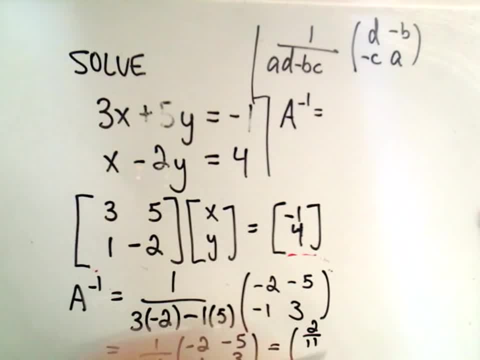 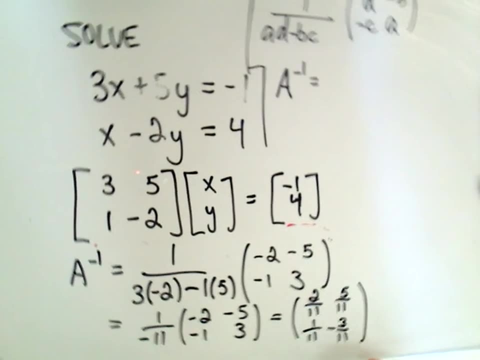 Notice this is equivalent to positive 2 over 11,, positive 5 over 11,, positive 1 over 11, and then also 3 over- excuse me- 3, negative 3 over 11,. okay, So that's sorry that all got cut off. 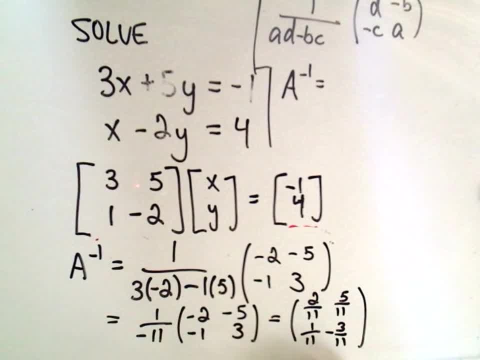 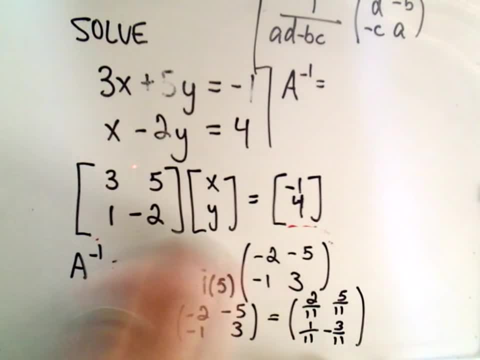 I wasn't paying attention here. So that's our A inverse matrix now, and that's the one that we needed. So let's see, let's erase all this for a second. So now what I have to do is I have to multiply both sides by the inverse. 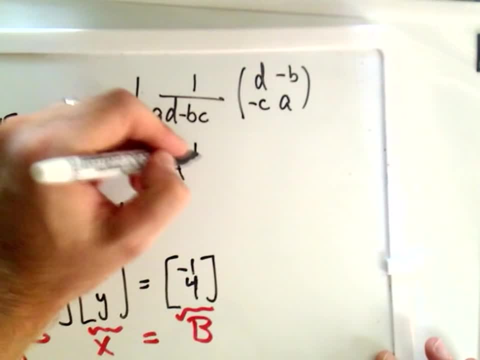 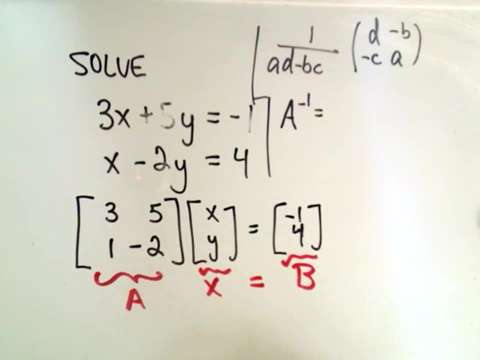 So in this case our inverse is going to equal. okay, so here's matrix A down here in the corner. Maybe we'll just see if we can't fit it all in here. So it says A inverse is going to equal. so I have to take 1 over 3 times negative 2,. 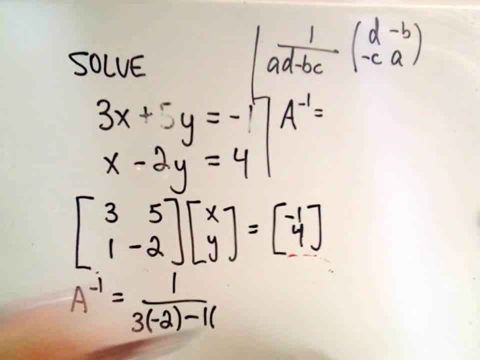 and then it says subtract 1 times 4.. 1 times 5.. And then I have to flip the 3 and the negative 2, so I'll get negative 2, 3.. And then I have to change the signs, so I'll get negative 5, negative 1.. 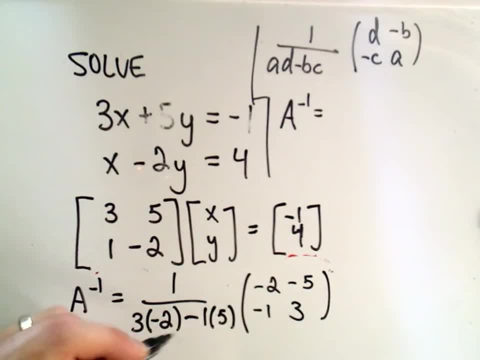 And let's see if we simplify this down, it looks like you get negative 6 minus 5,, which is 1 over negative 11, and then negative 2,, negative 5,, negative 1, 3.. Okay, 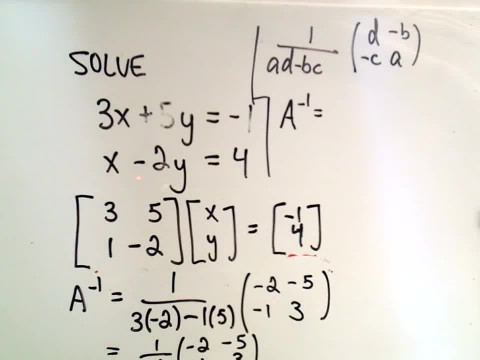 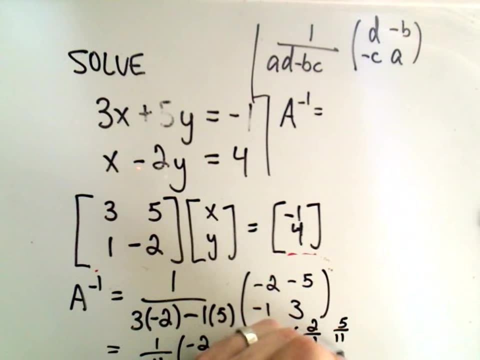 So that's our inverse matrix. We could go ahead and multiply this out and maybe clean it up a little bit. Notice: this is equivalent to positive 2 over 11, positive 5 over 11,, positive 1 over 11, and then also 3 over- excuse me- 3, negative 3 over 11.. 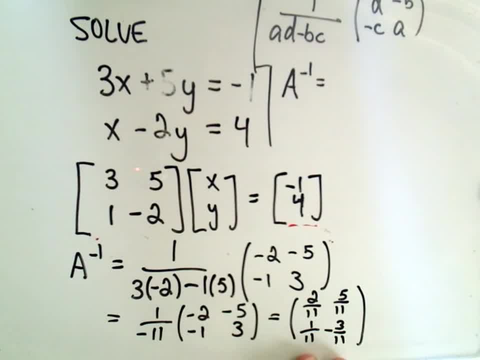 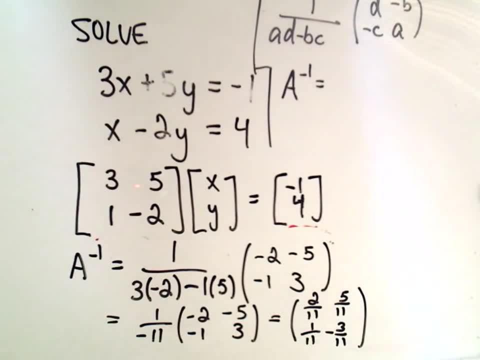 Okay, So that's sorry that all got cut off. I wasn't paying attention here. So that's our A inverse matrix now, And that's the one that we needed. So let's see, Let's erase all this for a second. 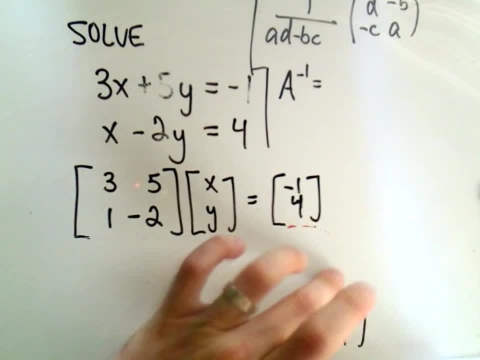 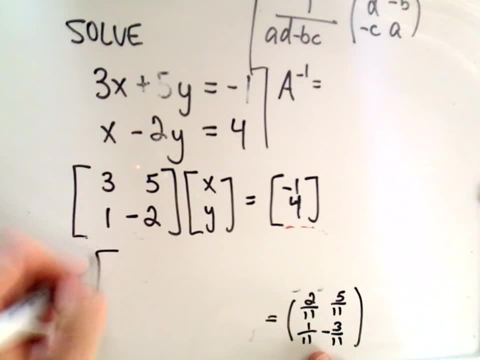 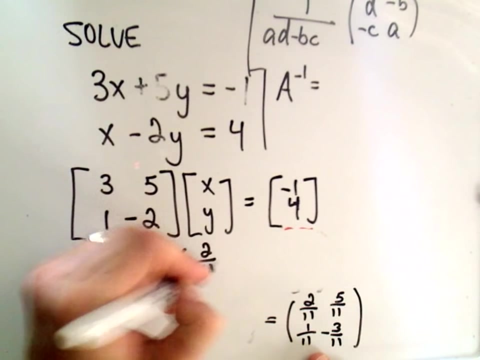 So now what I have to do is I have to multiply both sides by the inverse. But again, if you multiply the left side by the inverse, everything cancels out and you just get your solution. So we'll get x. y is going to be equal to 2 over 11,, 5 over 11,, 1 over 11,. 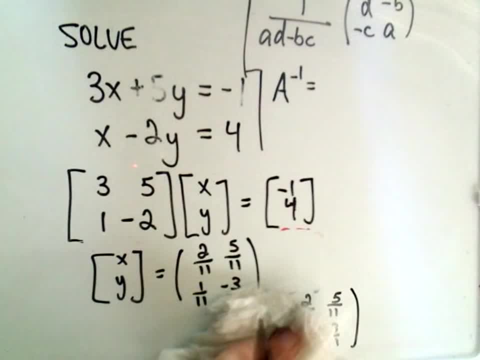 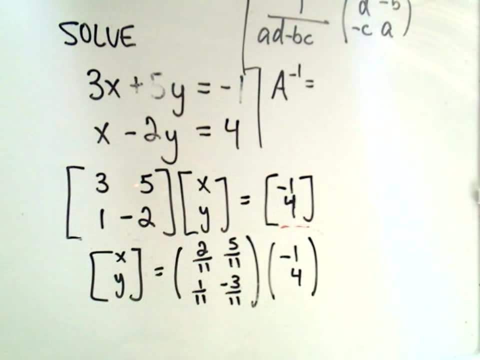 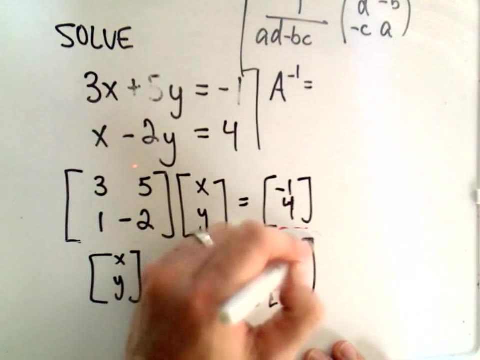 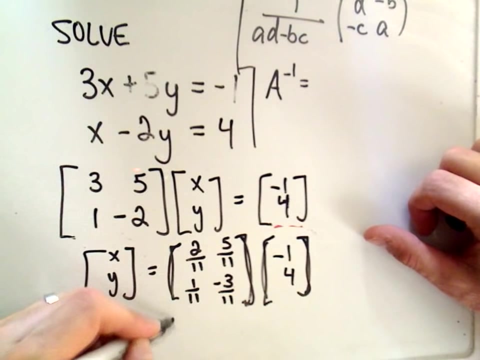 negative 3 over 11.. And now we need to multiply that by the negative 1, 4.. Okay, So my, I guess I should keep it here in brackets. It doesn't really matter A thing. to make the computations maybe a little easier is, I'm going to factor the 1 over 11 back out first. 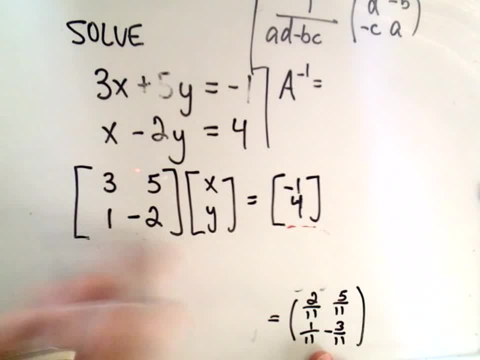 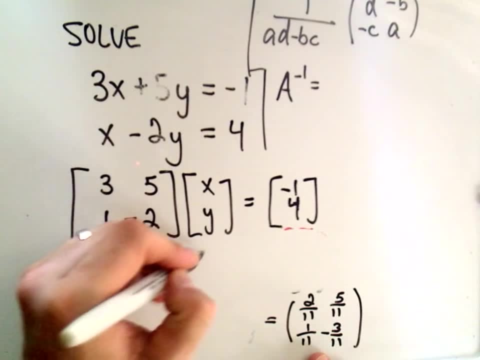 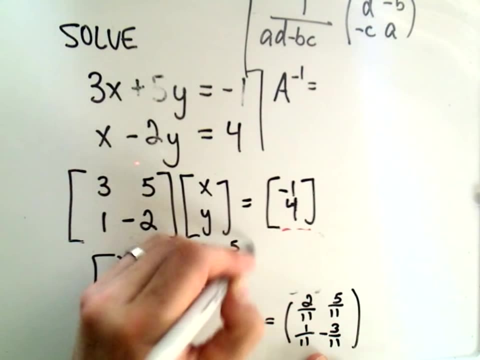 But again, if you multiply the left side by the inverse, everything cancels out and you just get your solution. So we'll get x. y is going to be equal to 2 over 11,, 5 over 11,, 1 over 11, negative 3 over 11.. 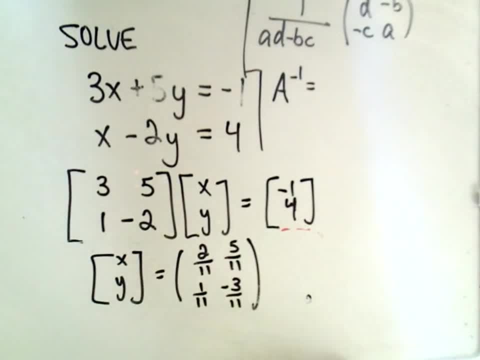 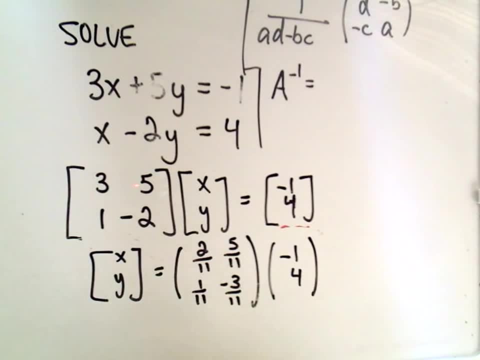 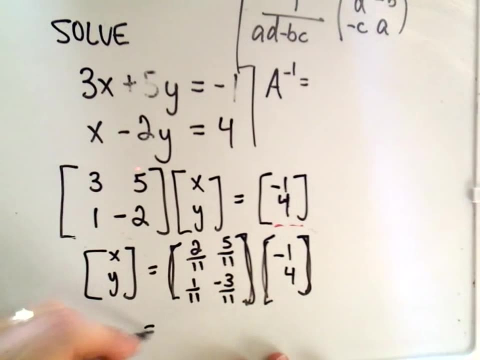 And now we need to multiply. We're going to multiply that by the negative 1, 4, okay, So my, I guess I could keep it here in brackets, It doesn't really matter A thing to make the computations maybe a little easier is I'm going to factor the 1? 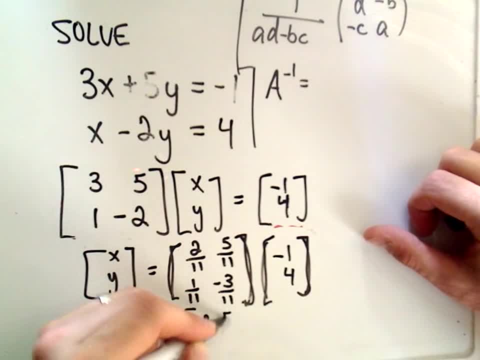 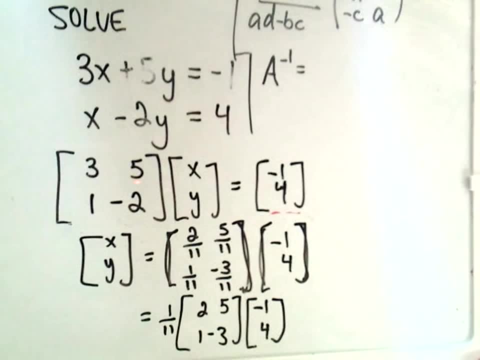 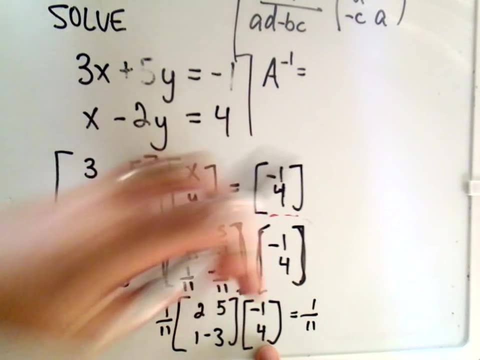 over 11 back out first. So then I'm left with 2,, 5,, 1, negative 3, and then I have negative 1 and 4.. Okay, so now if I multiply this matrix by the next one, I'll get 2 times negative 1,. 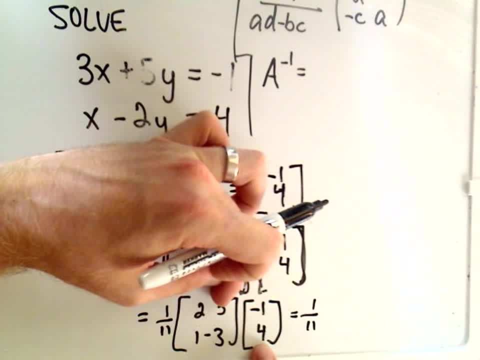 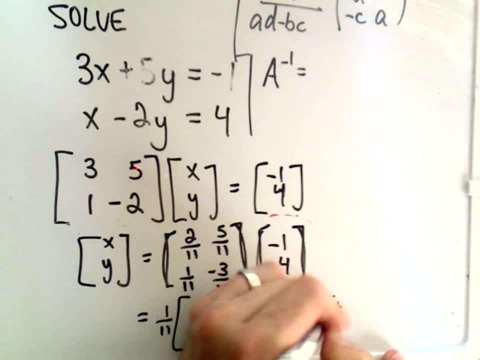 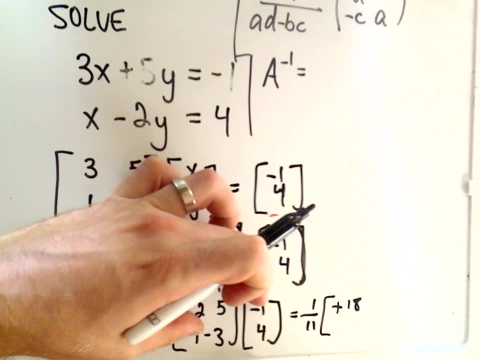 which is negative 2, plus 5 times 4,, which is 20.. So I'll get negative 2 plus 20, or that would be positive 18.. And then, for the next part, I'll get 1 times negative 1, which is negative 1,. 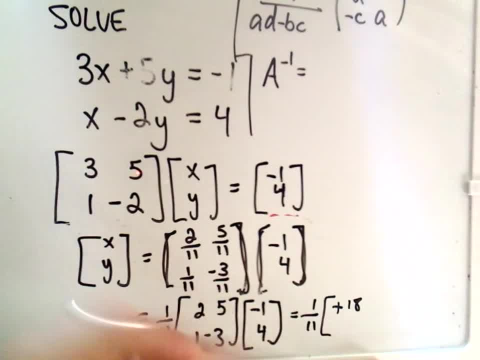 plus negative 3. which is negative 12,, so I'll get negative 13.. Or it says my solutions are: x equals 18 over 11, and y equals negative 13 over 11.. So kind of an involved little problem. 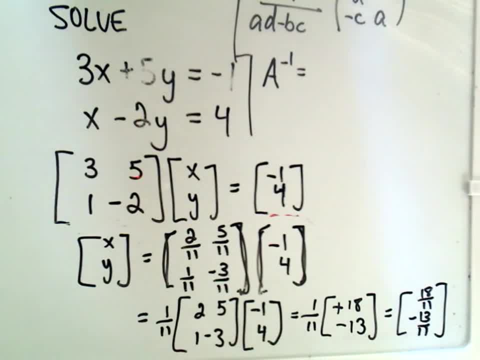 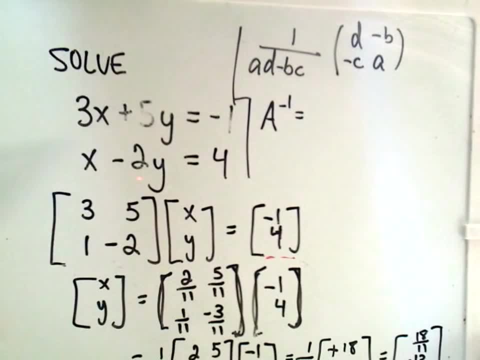 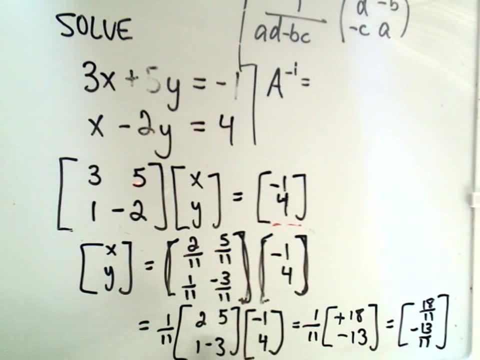 Sorry, I got cut off there for a second Again. the idea is you have to find the inverse of your matrix using the formula that we have up here. to get the inverse, Multiply both sides by the inverse, and whatever that works out to be, that'll be your solution. 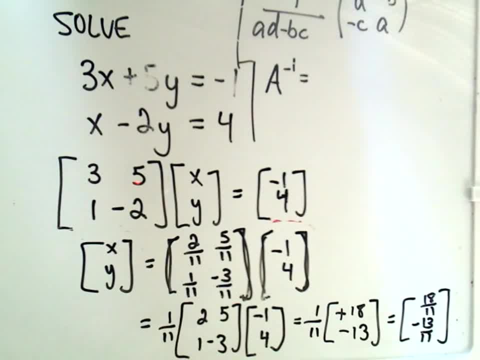 So again, I would suggest leaving this determinant just factored out front. I think it'll make the multiplication of the a lot of times the matrices a little bit easier. So I don't think I'm going to have time for another example in this one. 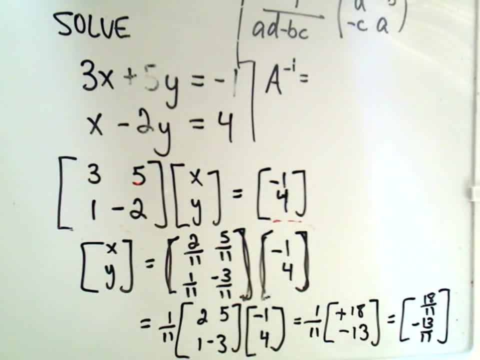 so I hope this helps. If you'd like to see another example of solving this type of 2x2 matrix using inverses, just let me know and I'll see you next time And I'll be happy to try to get another one out there.